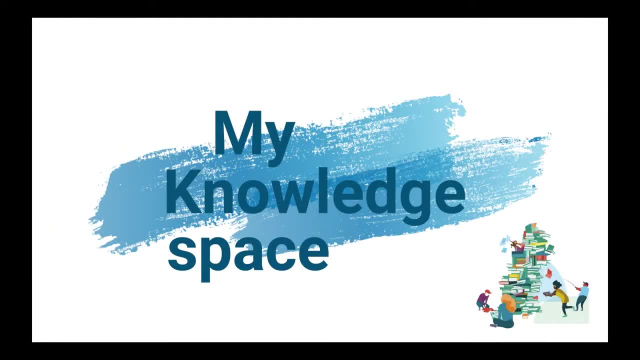 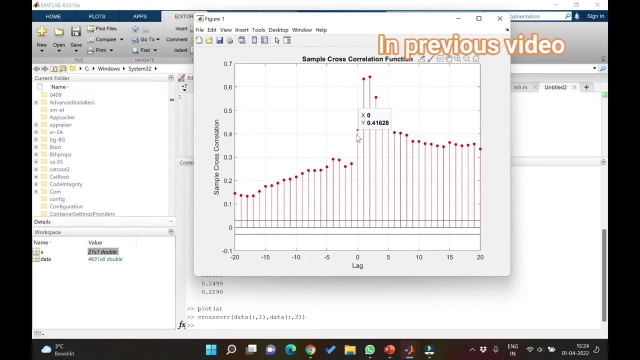 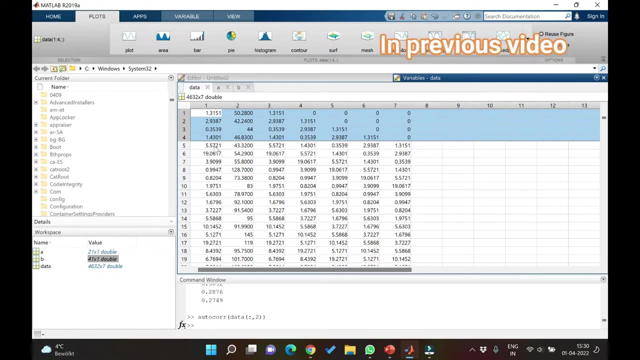 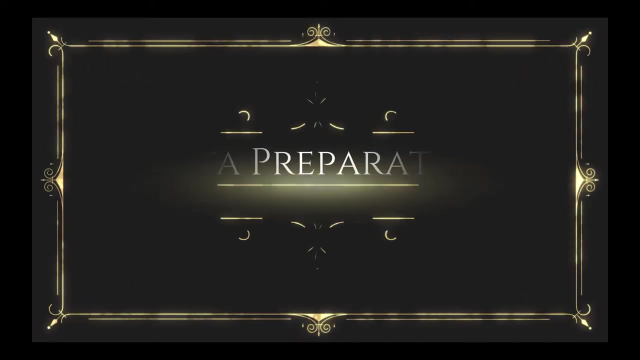 In the previous video we have seen the concepts about lag, autocorrelation and cross-correlation and also how we can understand the confidence limits and determine how many components we can use for developing any good hydrological model. In the current video we will see how. 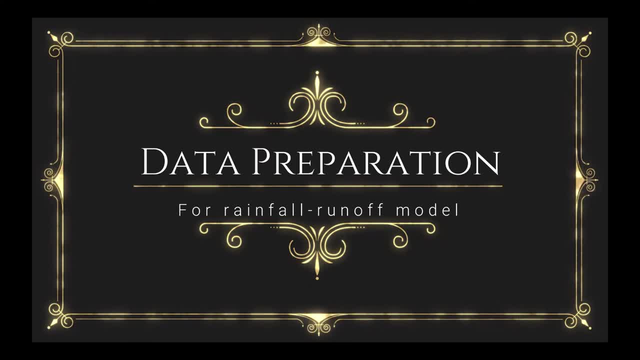 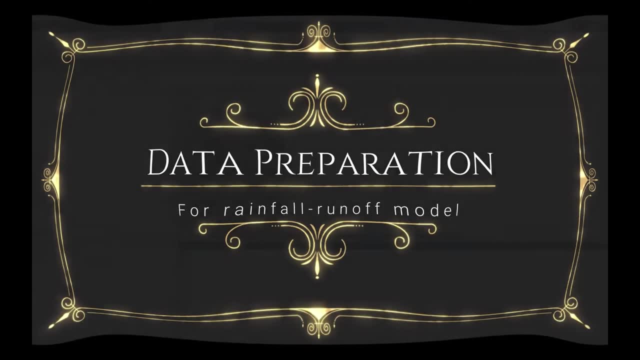 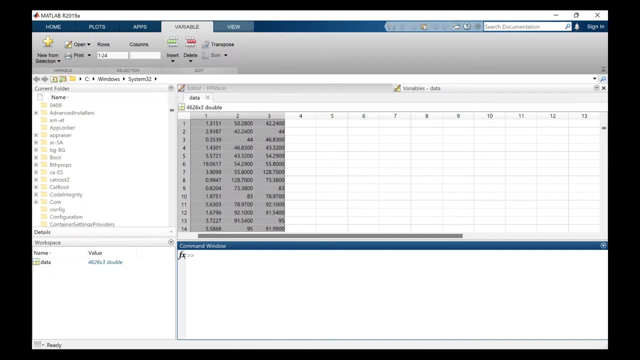 we can utilize those concepts learned in the previous videos and make data preparations for developing a good hydrological model. Hello everyone, welcome back to the channel. In this video, as mentioned earlier, we will see how we can make the data to use it for. 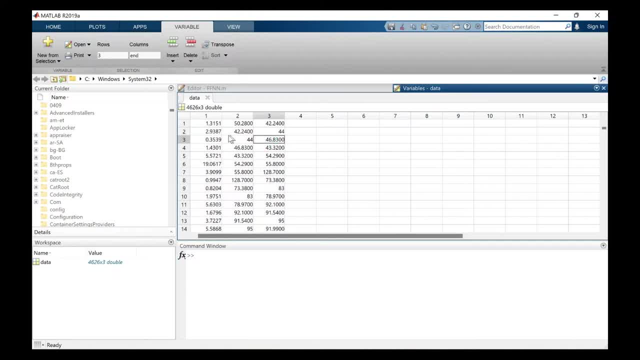 hydrological modeling. So, if you remember, the first column- we used in the previous video as well- is precipitation of a certain day, Discharge of a certain day and another column, data with discharge starting from the next day. So the first thing we need to know exactly to develop, to make the data to make a good 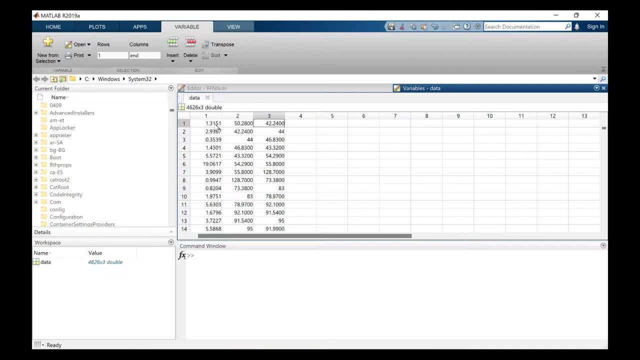 model is. you need to understand how many lags do we need to do to the data to have good information. in itself, The model can understand the trend. You can directly use these two data and put this as an output in a linear regression model or an artificial neural network model and can. 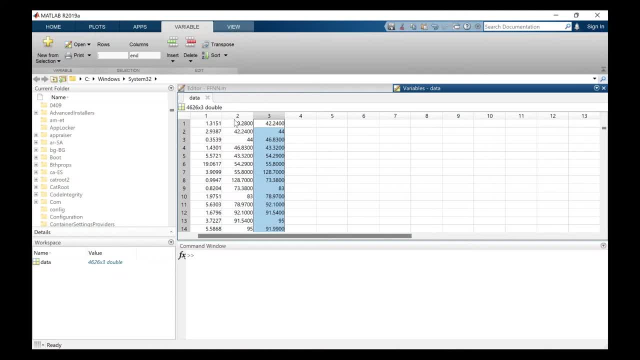 develop a good relationship and get good results. This model predicts one day ahead discharge because, as you see here, this is, let us assume, the first January of 2021. discharge. we are asking the model to predict the second january discharge, so to understand this, we. 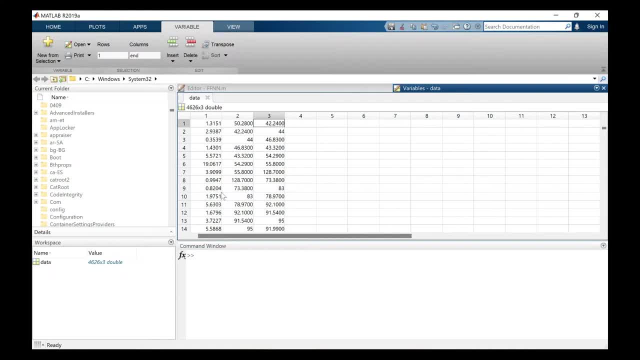 need to get the lags so as if you have seen the earlier video, i have shown you how the lag components can be obtained using auto correlation and cross correlation. if you have not yet watched it, you can watch the video in the description. if we see here we find autocorrelation, so we are. 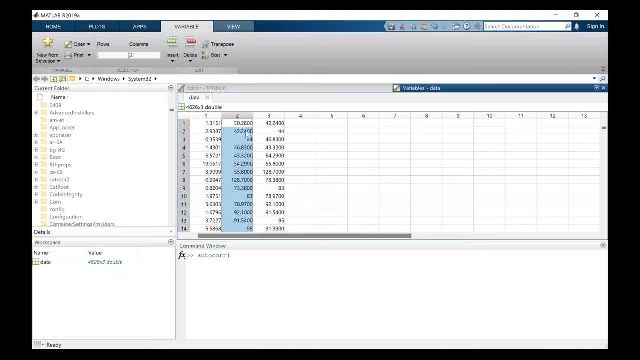 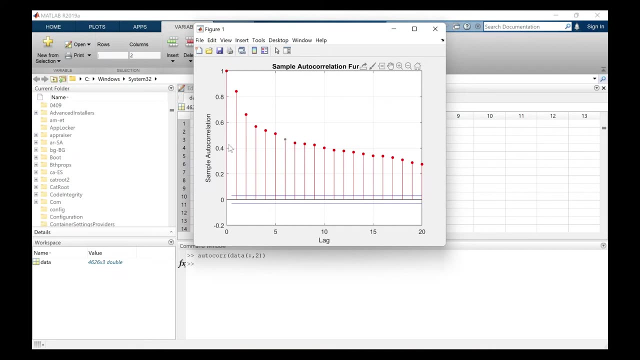 trying to predict discharge. so we will see what is the discharge. autocorrelation, again, we have already discussed it in the previous video. so you see, we will take a confidence limit of 0.4 and see how many variables are above 0.4, so that 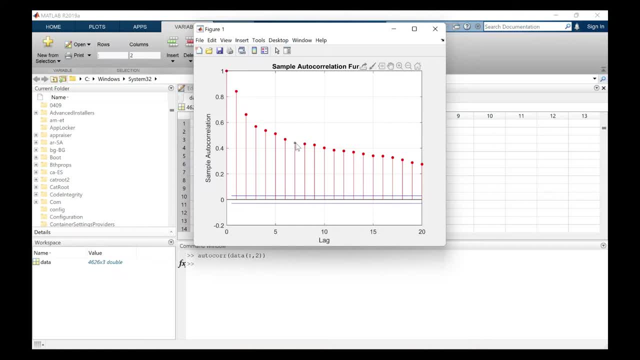 we can use them for preparing the data. so if you see, here there are up to 9 variables and almost 10 variables are there, but i would like to take a value greater than 0.5 in this case, just to have lesser variables. to explain it to you, 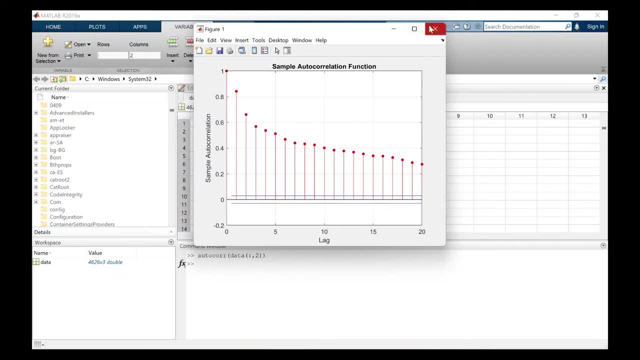 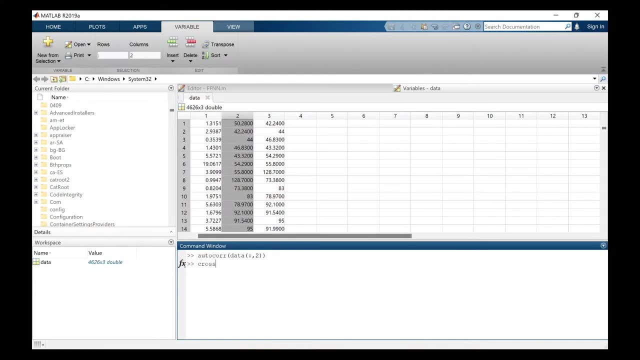 so we will see we have to take 5 lags for discharge, let's remember that- and we will also see correlation which tells us how many precipitation lags can be used for getting a good model. so the first column is precipitation, second is discharge, and we will see the thing. 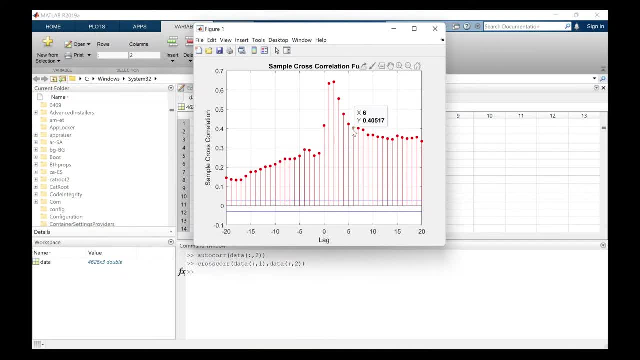 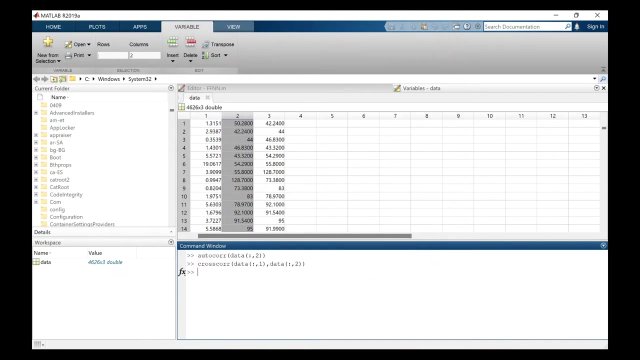 and here again i will choose a value with greater than 0.40. so i will be taking again here five lag values to develop the data so that we can get good model. so, as you have seen, the discharge and precipitation lags are five and five. let's go to excel and see. 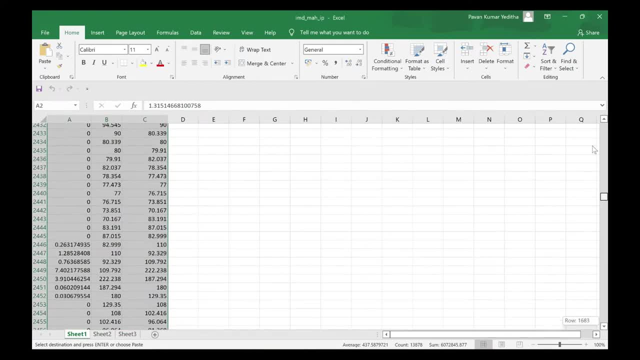 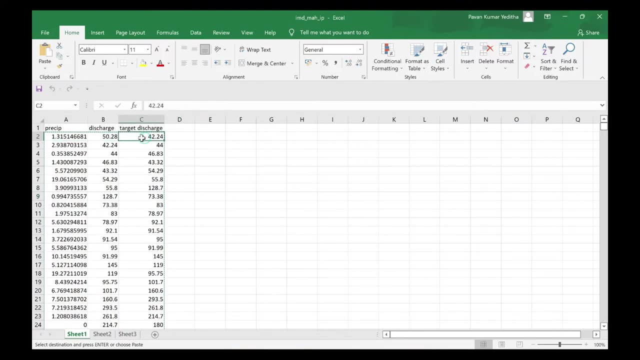 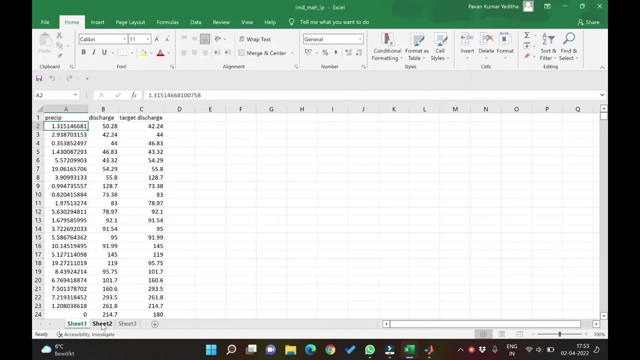 your data and make the data so that we can use it. so, as mentioned again, today's precipitation, today's discharge and tomorrow's discharge. so now what we need to do is do lags. so let's see how these lags can be done. i have already put the lag data. 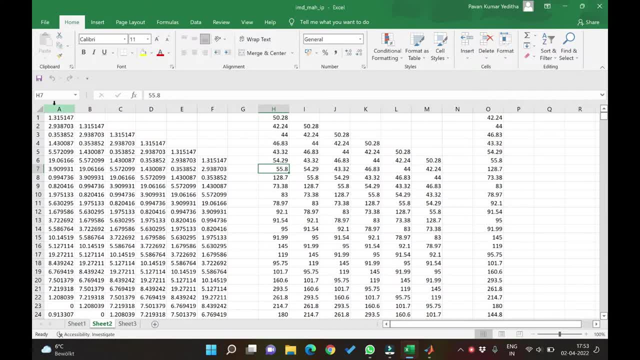 in the sheet so that i can explain. so the first column is the original set, which we can also term it as zeroth lag of precipitation. when we leave one row here, then it becomes one lag, this becomes two lag, three, four and so on, similarly even discharge. 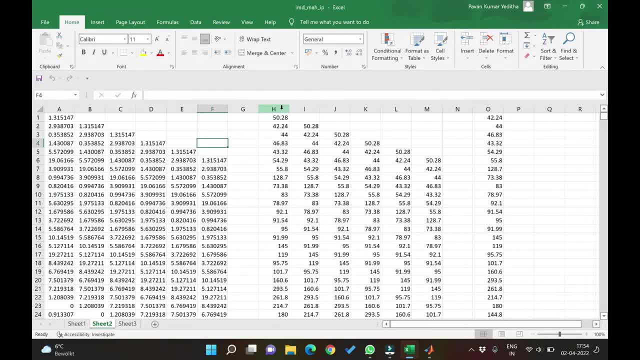 as we saw in the plots earlier. it is also we wanted it to take five legs. similarly, it will become zero in flag one, two, three, four and five, and this is the target data set if you see the next day value. so now, if you see, here we are having 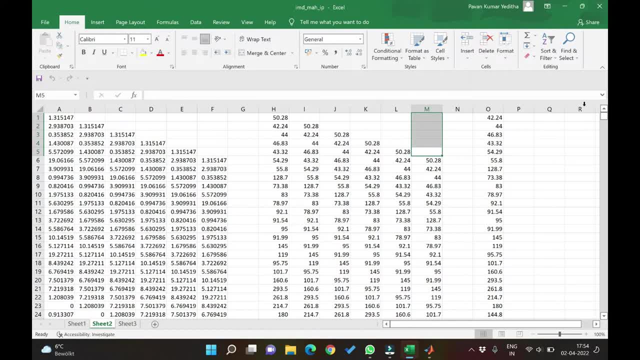 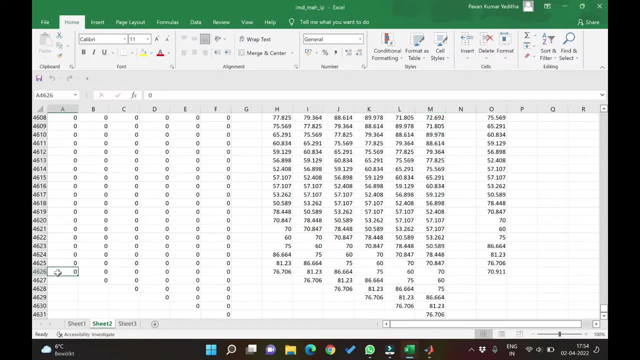 empty rows here, empty rows here and also in the below. at the end of the data you will have similar phenomenon where you see this should have been the original length, but because we are taking lag, this data is excess. So what can we do about it? because we cannot just. 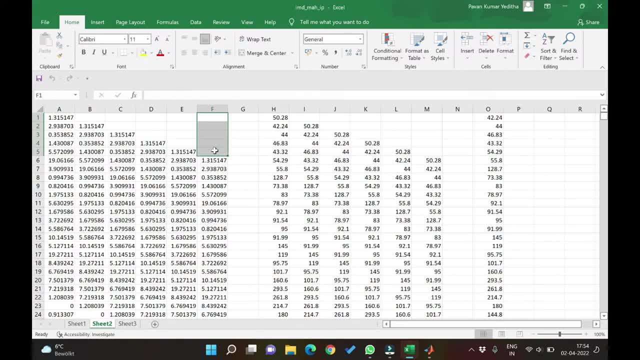 directly use this with zero values as inputs. So to do it in a correct way, one method is to remove the first five rows in all the elements, including the inputs and targets, as well as at the bottom also. So first we'll see how we do at the top, If you see here when we try to remove all the data. 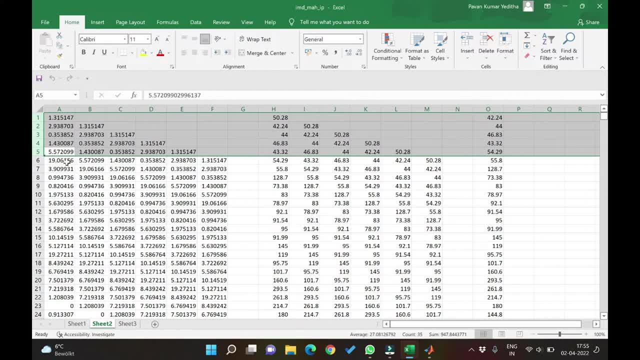 sets. here we are getting a value of 19.. So if we think 19 is today's data, so we should have one data of yesterday. if we are taking one length, lag right. so if you want yesterday's data, so it'll have yesterday's component in two days. 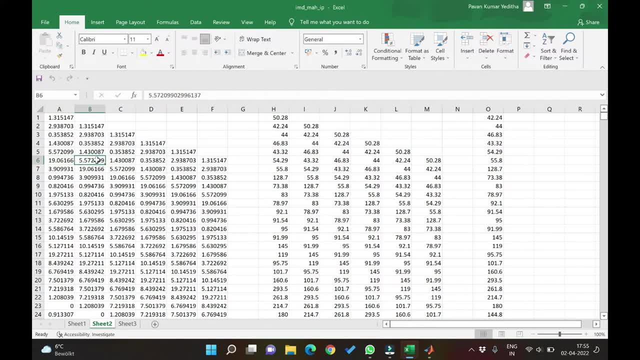 so if you see the value of one lag here, you see there is one value already before the 19, which you can already see here. this becomes one lag where you have one data before two days. when you go to this second lag, you see there are two datas after we remove these things. similarly, here we: 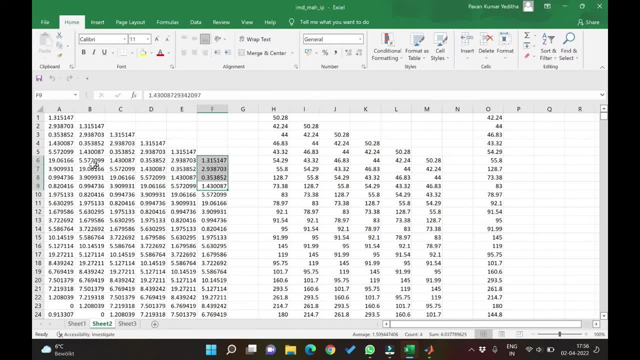 have three, four and five right. similarly in discharge, if this 54 is two days, then 43 is yesterday's, 46 is day before yesterday, and so on until five days before. if you see here 54, 54, 54 is today's 43, 46, 44, 42 and 50, that becomes the data of five days before 54, even after removing. 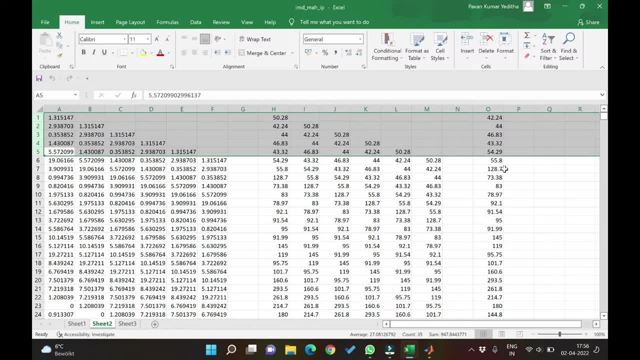 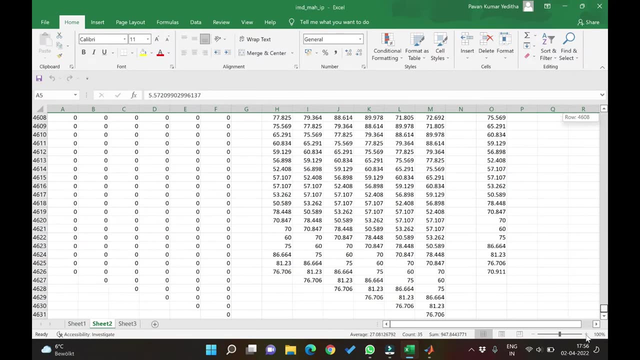 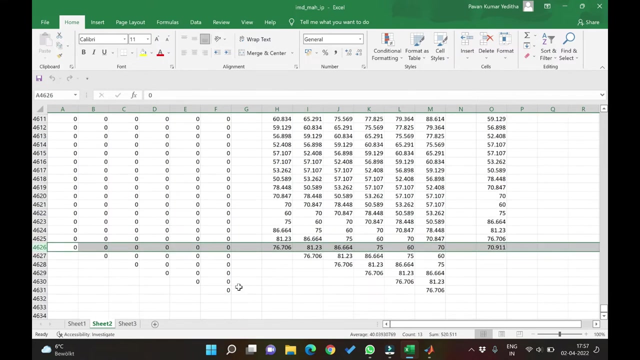 these five elements, you can see the target of the data is 55.8, which is the next day after 54. so this is how you remove the first five components. when we come to the last five components, after adding this directly, you just remove it without any issue, because they are all excess data. 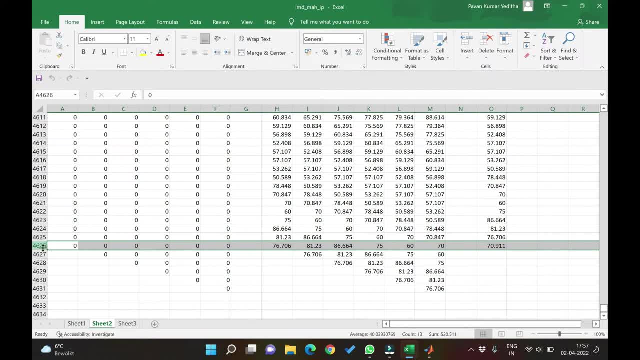 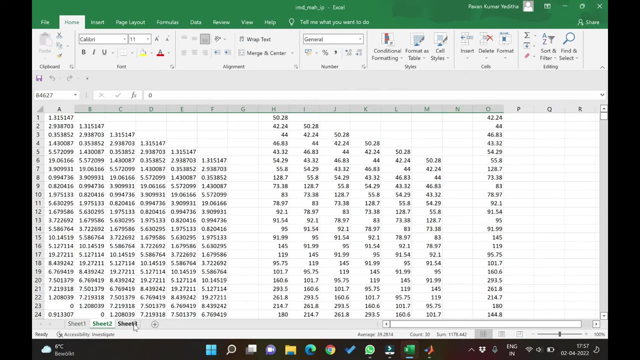 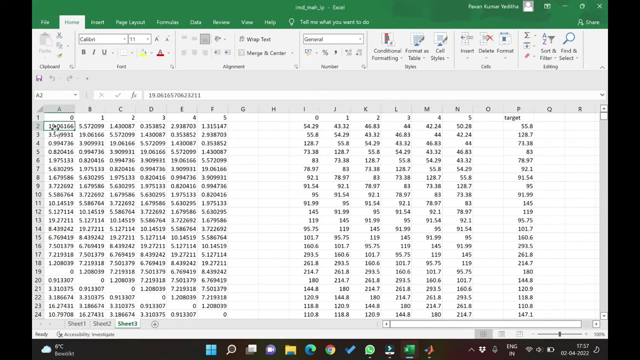 and you have the original length again here after removal of all these data sets. so this is how you remove the data. so let's see what will, how the data looks in a clear way after removing. so if you see here, as i have mentioned earlier, this becomes our original data after removing the first five rows. 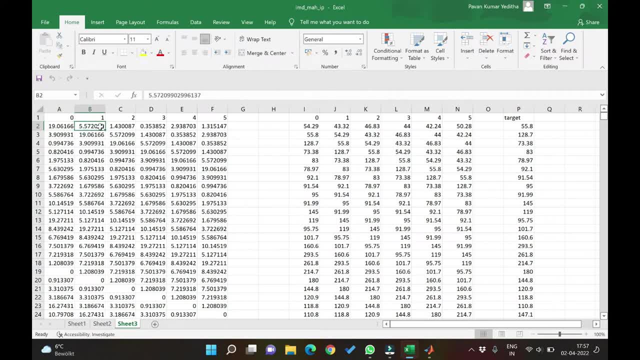 this becomes the first lag, having one day before our day, this two, two days, three days, four days and five days before our data, which we want to analyze similarly for the discharge as well: one day, two day, three day, four day and five days. so this is how we can put lags for precipitation and discharge without causing 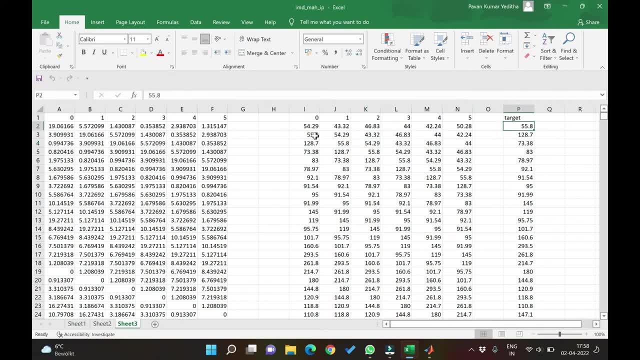 an issue or prediction of tomorrow's data. you see here, tomorrow is 55.8. that is what we are trying to predict. so now what we can do is we can just copy all these data, these five rows here, these five rows here, and we can just copy all these data, these five rows here, and we can just copy all these. 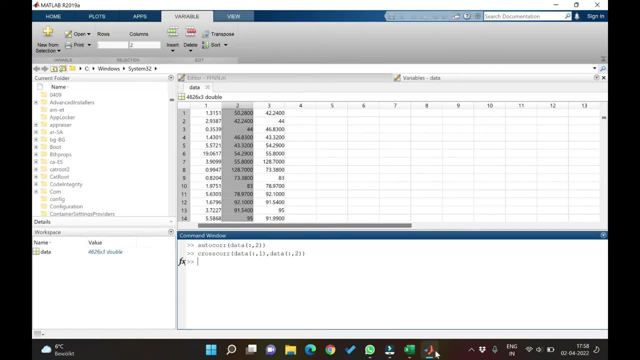 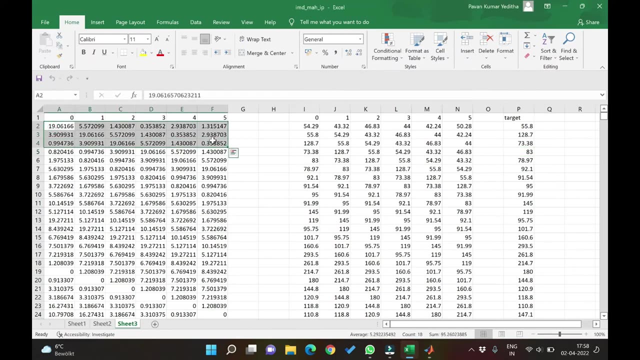 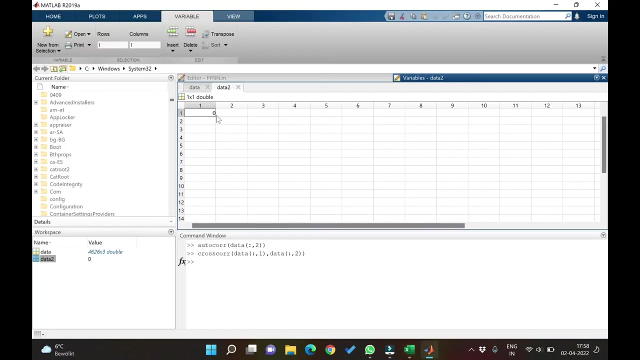 data here and this one into MATLAB and make the data in MATLAB. we can term it as data 2, and what we can do here is we can just ctrl shift lower arrow key, long arrow, and we can copy all these a key elements, page them here, then again control shifting lower arrow keys, then again paste them.